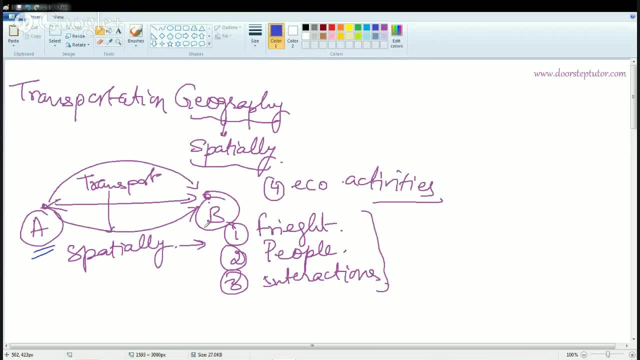 the reasons for connectivity between points or city A and city B. So when we talk about transportation geography, we must understand that through civilizations or historically, the transportation has grown and developed and there were important centers that started to get connected Slowly and gradually. there were main transport arteries. 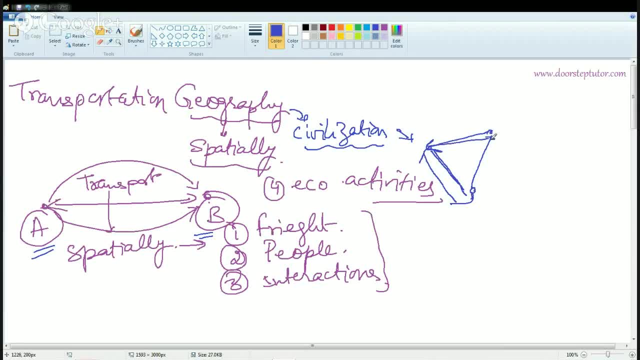 that were found between those regions, which were strongly connected, and there were less development or less arteries between the weakly developed regions. So the important impact of transportation is because of civilization. then you have social and economic reasons because of which transportation has been taking place Under transportation geography. 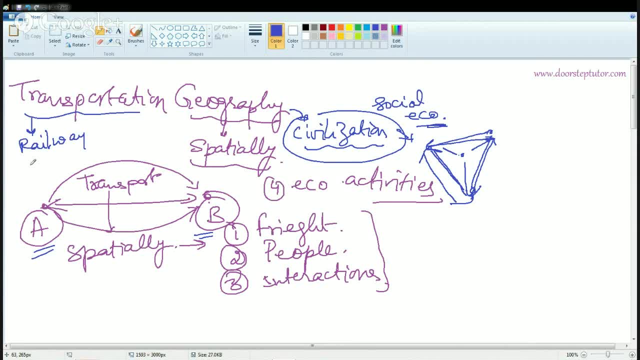 broadly, we include the various forms of transportation, ie railways, roadways, air transportation transport, ship or water transport. Now, to understand the concept of transportation geography, there is one concept that we must and will try to understand, and that is the concept. 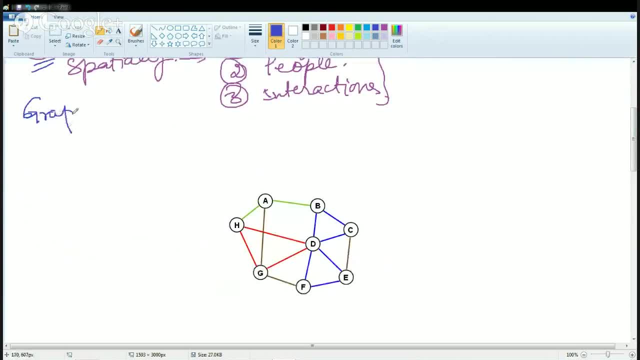 of graph theory. So let's start with what is the concept of graph theory and what is graph? So, when we talk about the encoding and measurement of any network, that is what is graph theory. So it's simply a function of V and E, where V is the vertices and E is the edges. 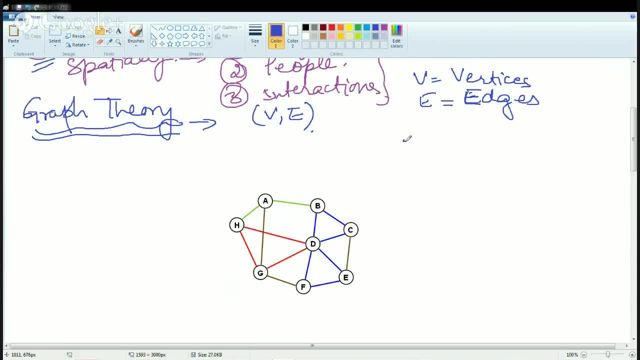 Now, if I say, let's take a very simple example, I have two points. one is Los Angeles, other is the city of New York. So these are the two vertices and this is the edge that is joining the two vertices. So edge is also known as link and vertices is also known as a node. 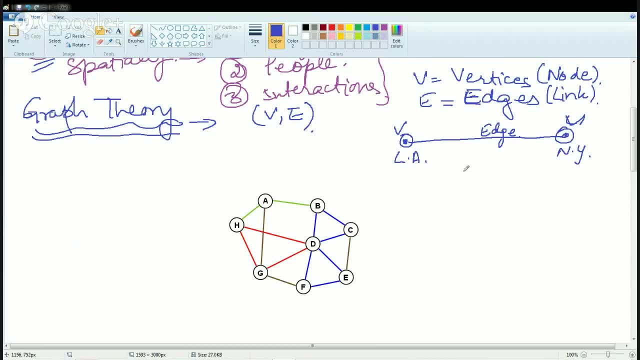 Now let's look at the graph. What is the size? So the number of edges that we are talking about is the size. So if I say there is just one edge that connects Los Angeles to New York, however, in practical situation this is not the case. I am just taking an example. 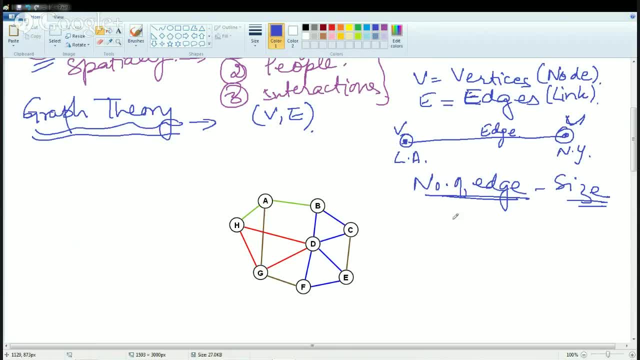 So that would be the number of edges, would be the size. Now I will help you understand the remaining terms with the number of edges. Now in this diagram, as you can see, there is a green line which connects edge A and B. So this is a kind of complete graph. we can say: edge A and B. 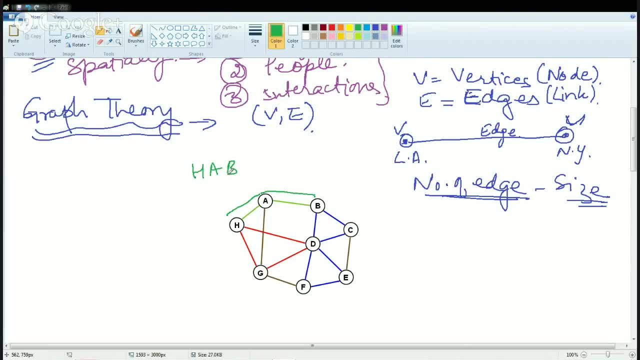 So this path, this point which connects edge A and B, is a path. Now there is a term called as walk and there are two kinds of walk: open walk and closed walk. Open walk means if I start, open walk is basically a path. so I am starting with edge and moving. 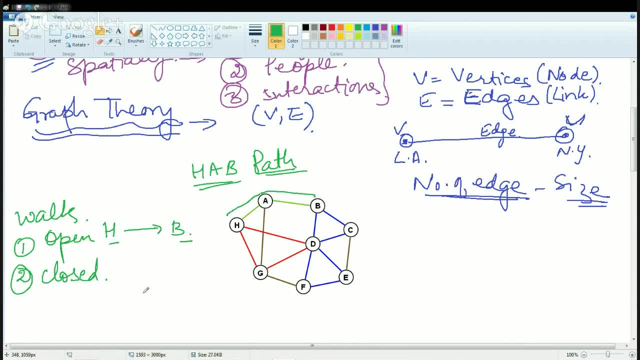 on to B. So my starting point and ending point are different. so that is the case of open walk, The next is closed walk. Closed walk simply means if my start point and end point are same. So, for example, if I go from edge A, B, D and B to edge, 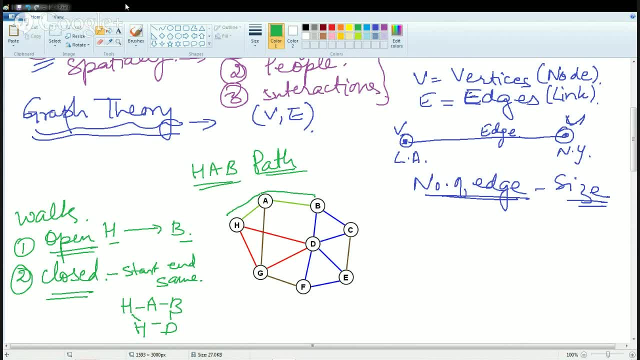 So that would be a kind of open walk. But again, if I take the same example- edge A, B, D, H and from there I go to G and come back to edge, that is my final location, So that would again be a kind of closed walk. 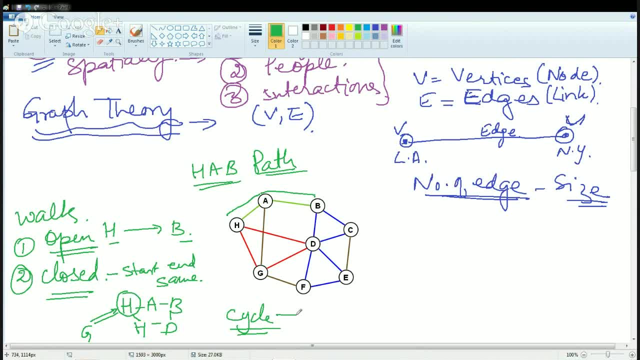 But in case of cycle or a simple cycle, what happens is there is no repetition of edges. So if I start with H, D, G, So that would again be a kind of closed walk. But in case of cycle or a simple cycle, what happens is there is no repetition of edges. 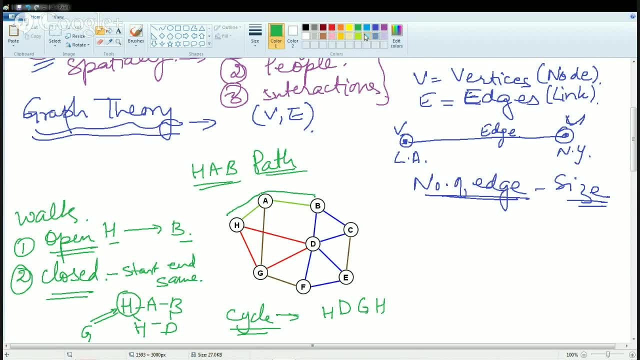 So let's take H, D, G and H, those marked in the red. So you have this, this and this. So what I am doing, I am coming back, starting and coming at the same point, but no repetition of the edges. 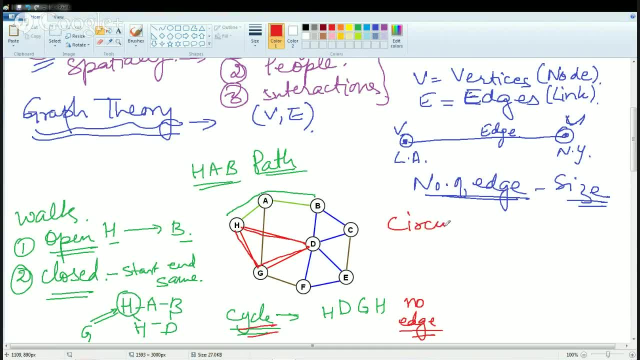 So that is what is a cycle. Now, what is? circuit Under circuit, you have repetition of vertices. Okay, So this is a cycle. So what is a cycle? So here you can say: I am starting from D, B, C, D, E, F and back to D. 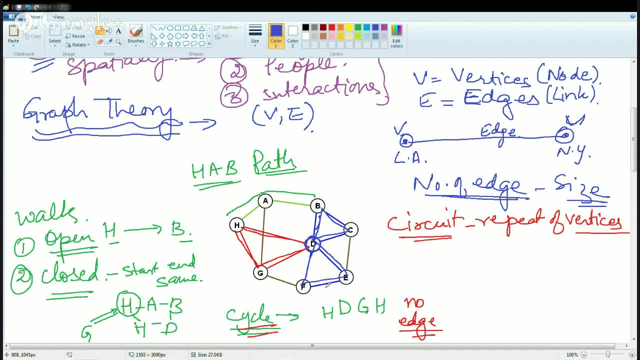 So, basically what is happening, D is a vertex that is being repeated. There is no repetition of H, but there is repetition of vertices, And this is what is known as a circle. So, under graph theory, what we have tried to understand today is: what is a circle? 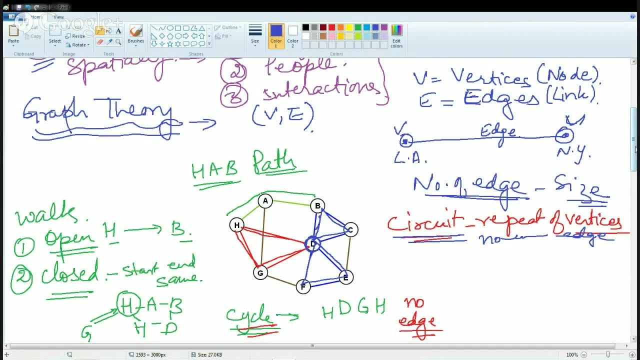 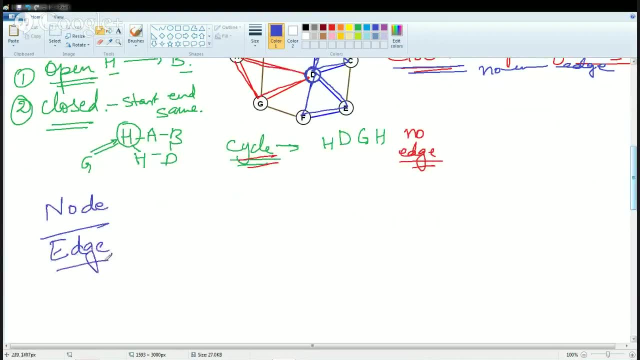 What is a circle. So what we have tried to understand today is: what is node? First, node or vertex. Then we have talked about edge or link. We have talked about two types of walk: the open walk and the closed walk. We have understood the concept of cycle and circuit. 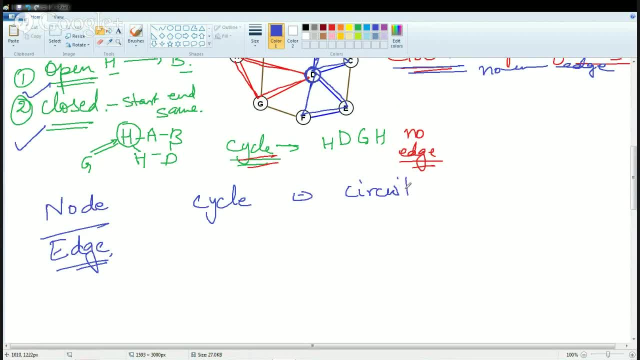 So cycle and circuit, the difference is very important. Okay, Now there are a few things that you must know. under graph theory are the connections in the graph, so connections in graph. so first kind of connection is walk, we already talked about. the second important connection is: 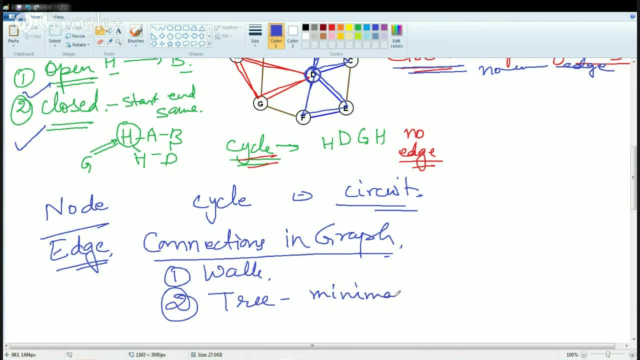 tree. so tree is minimally connected graph, which implies that there is only one possible way to reach any point. for example, I mark point A, B and C- okay, and then you have D, okay. so there is only one way to reach to C and there is only 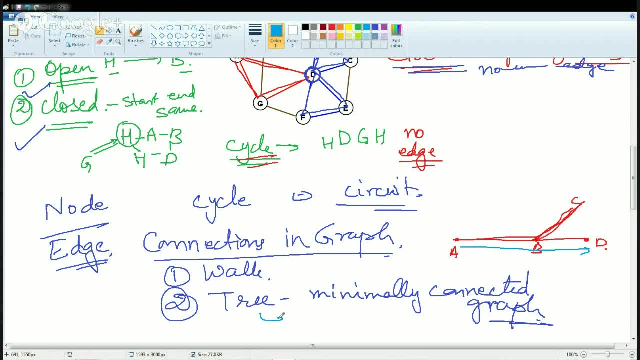 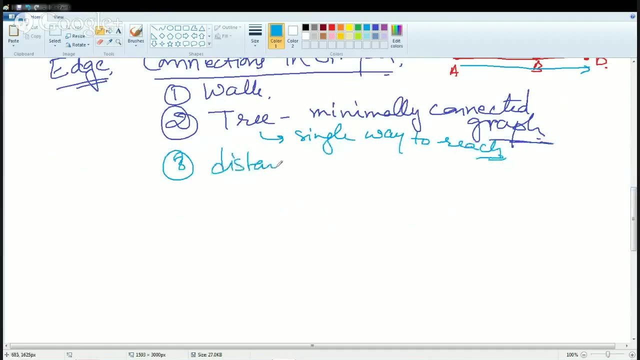 one way to reach to D. so there, when there is a single way to reach to any place, that could be the tree, okay. the next connection here is the distance. so distance is basically between two vertices. so this is what I say and this is what has been, so how far. 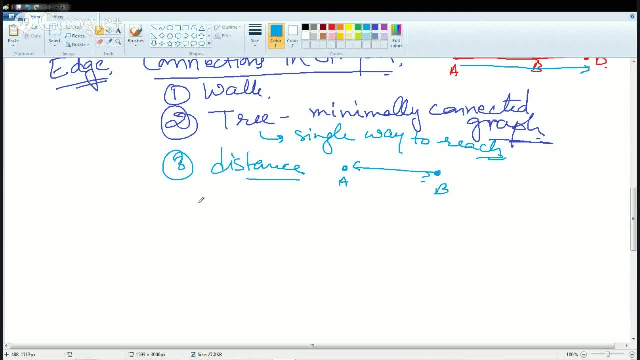 they are would be the distance. then you have the length. so length is the number of ages, so length is basically: how many edges are there between the various vertices? okay, so that will be the edge then. okay, so that will be the edge then. okay, so that will be the edge then. 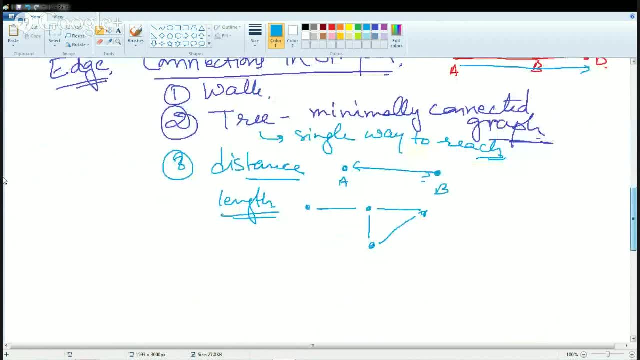 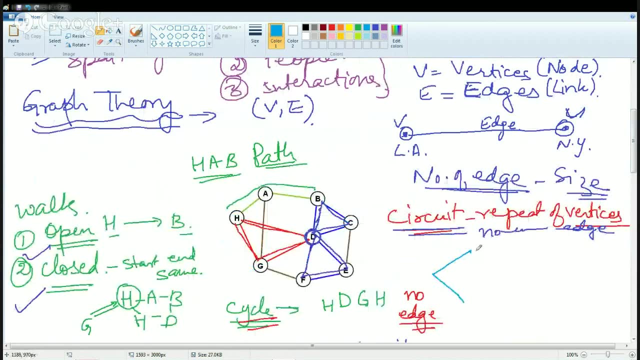 just come back to this graph here and I'll try to explain you the concept of chord. so if I draw a diagram here, okay, these points are connected to the essence, but point that is not directly connected would be the chord. so this is what is the chord. now you have two important 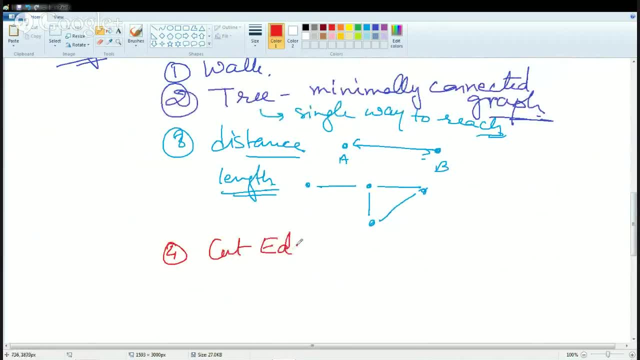 terms, that is the cut edge. cut edge is also known as bridge or isthmus. now, what is a cut edge? for example, I have a graph here, okay, and they say: this is connected in this fashion. now what would happen if I remove the this edge? this point or vertex would get disconnected, and so this graph would. 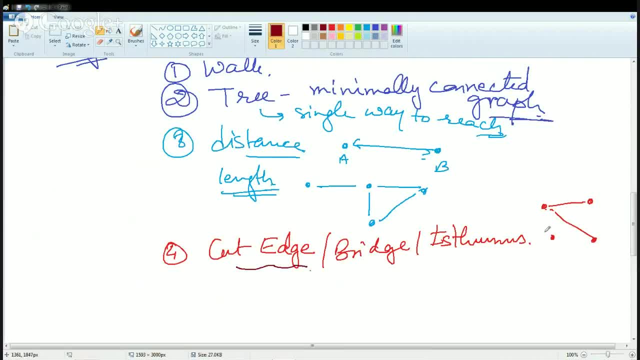 become disconnected, and that is what is a cut edge. so this vertex becomes independent and disconnected from the rest of those. so one removal of one edge disconnects the graph. the next is cut vertex. so if you have three points here, okay. so if you have three points here, okay. so if you have three points here. 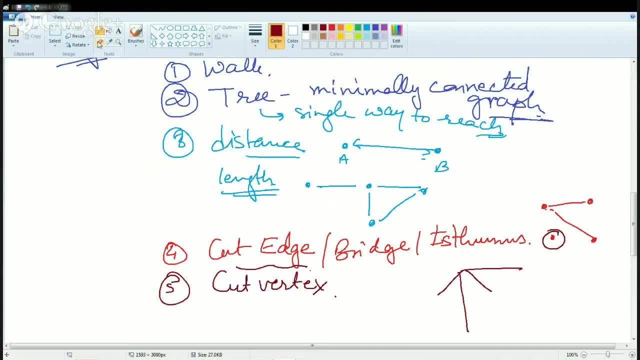 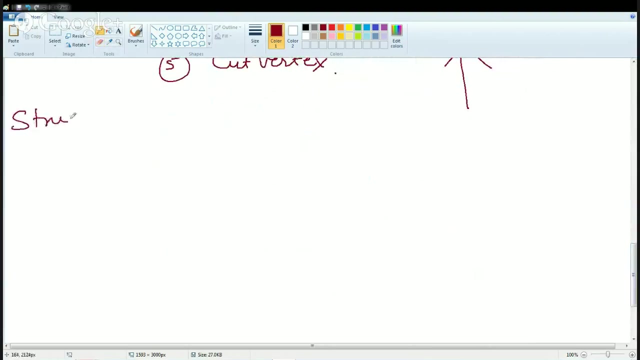 okay, and I cut this vertex or I remove this vertex. okay, what would happen is there would be a kind of our disconnection in that sub graph. okay, now, these were the general connections in the graph, so let's talk about. the next thing is that is the structural property. so structural property of a graph, and 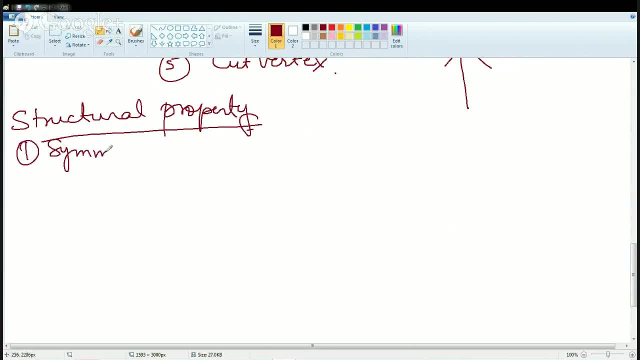 structural property. first is symmetry, or asymmetric symmetry means all the edges and vertices are linked in one direction. so that is kind of symmetry. the next is connectivity. that means one vertex is connected to another vertex. okay, that is connectivity. the curve is complement. now what is complement of a graph? so